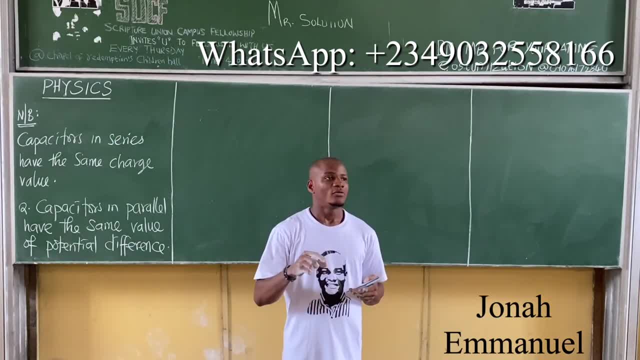 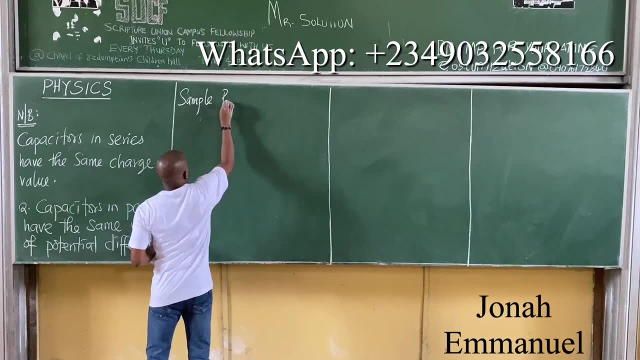 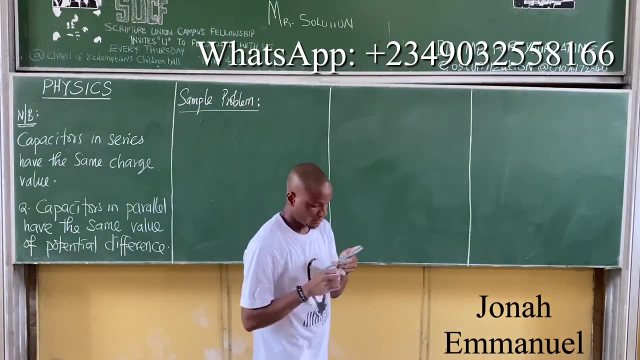 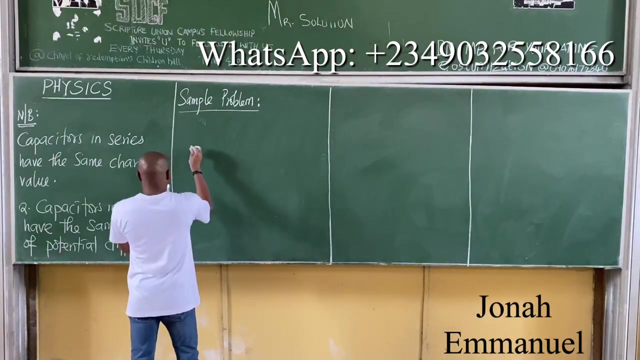 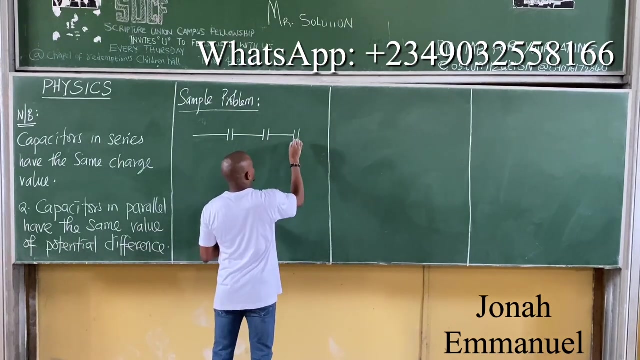 value: Sample problem. Sample problem. For the next function below sample problem. The next function below: Sample problem: Low Low. For the network shown below: find the equivalent capacitance comma. find the equivalent capacitance comma, the charge and the potential difference across each capacitor. 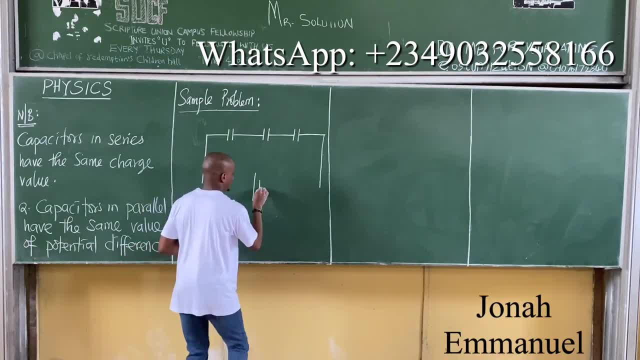 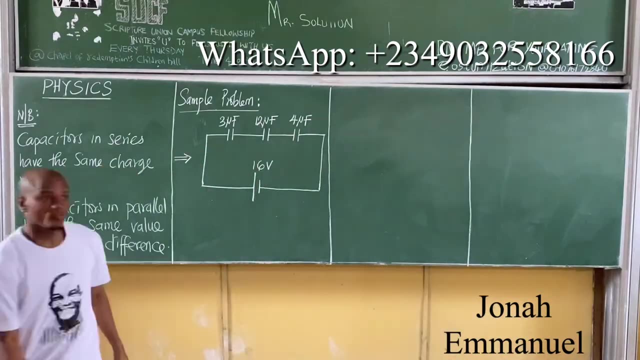 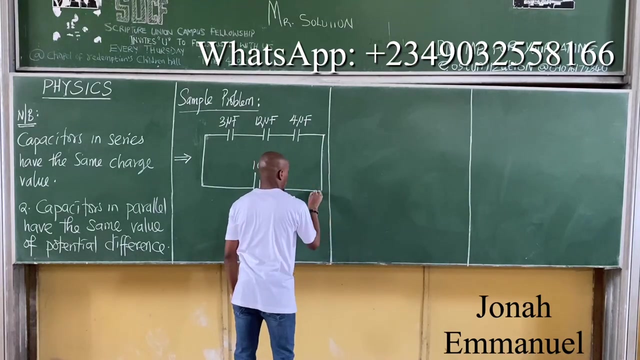 the charge and the potential difference across each capacitor, as shown in the notes. Now, listen up, Listen up. If you have some problem with this, listen up. Your first task is to get C1, C2, C3.. Now, mind you, they didn't give you a value for C1, C2, C3. 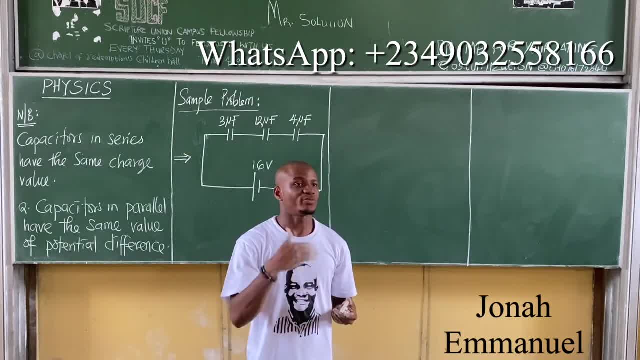 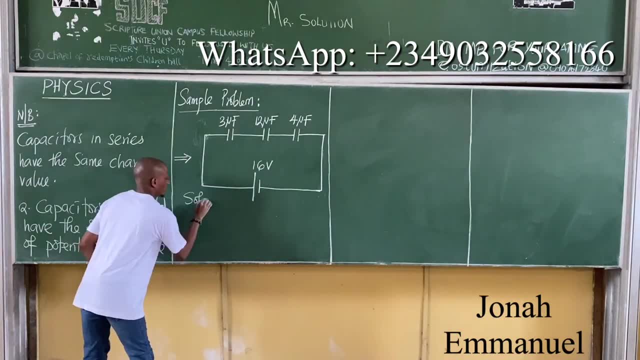 So which of them should be C1?, Which should be C2?, Which should be C3?? Please use any one, Right? So my first solution, I'll say: let C1 be equal to this Three microbarons. C2 will be equal to this one here. 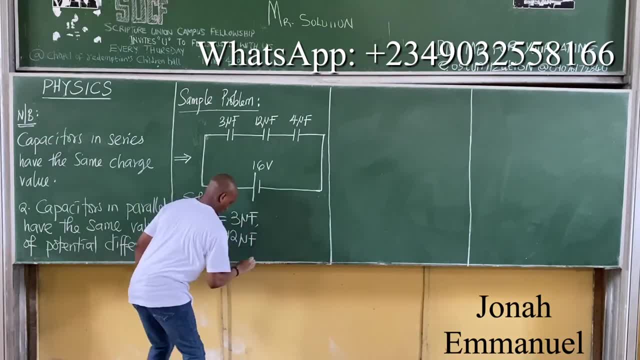 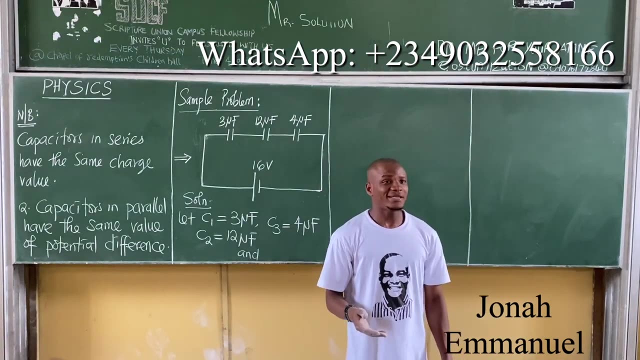 So what I'm going to do is four microbarons, and C3 will be equal to four microbarons. Now here's the thing. So I'm first going to say solution: C1 plus C2 plus C3.. The idea is this. 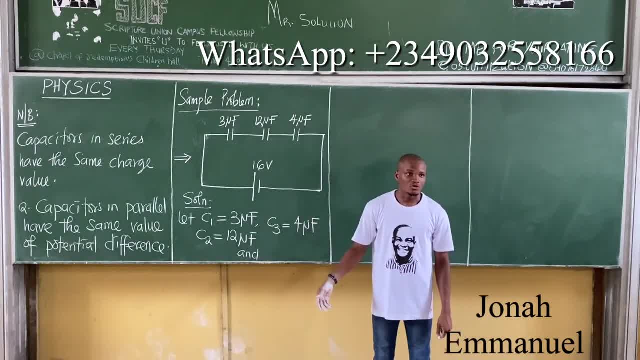 In your question you are not given C1, C2, C3. So you can't just go on and start saying C1 equal to this. No, You have to go on there, define them first. So I'll define them. 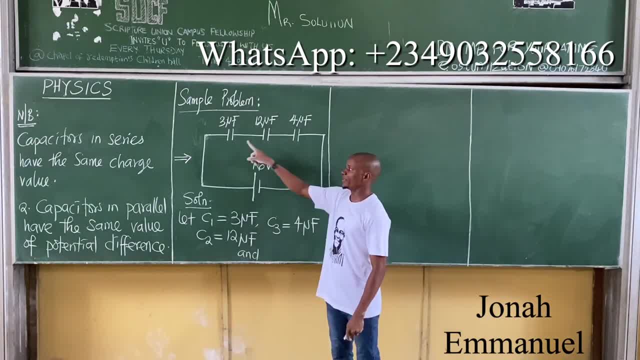 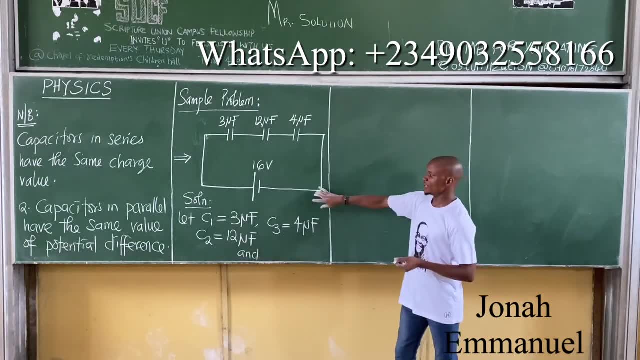 If you choose to say let C1 be this, C2 be this, C3 be this, it's still correct. First I'm going to find the equivalent capacitance. Of course, this is series arrangement for this one here. 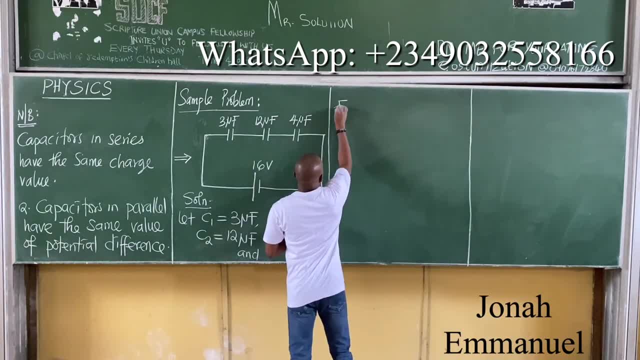 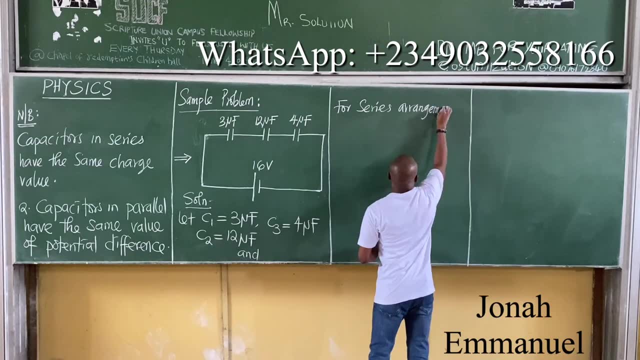 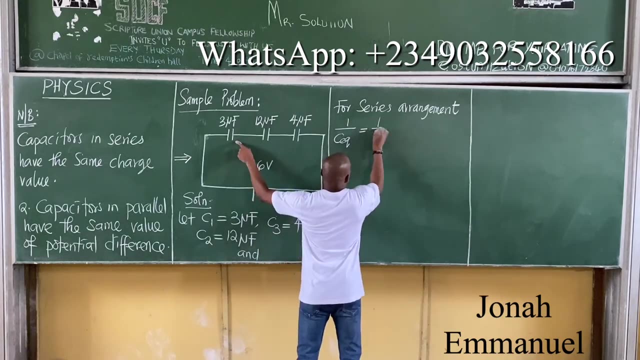 This is series arrangement. So for series arrangement, for series arrangement, what I have is this: I have that the equivalent capacitance is equal to one over. We call this C1. So C1 plus this one here, One over, C2 plus this one here. 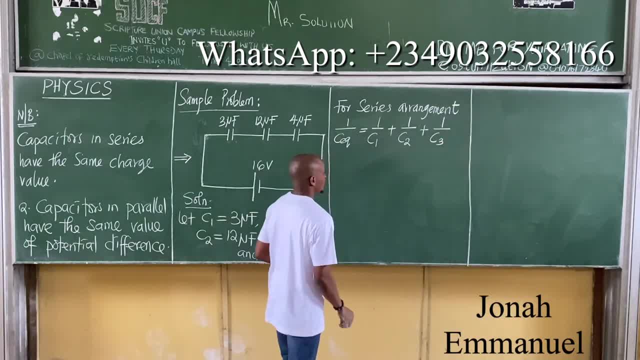 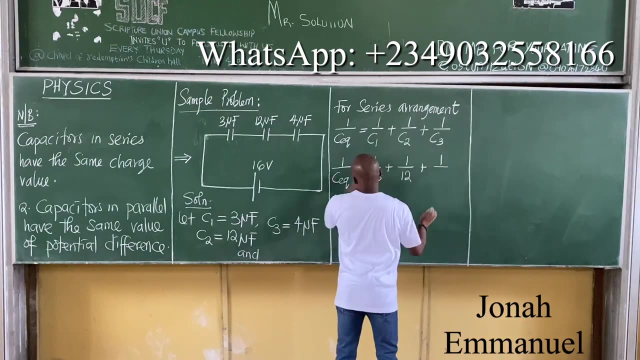 One over C3. In this value I have, one over equivalent capacitance has been equal to one over C1 is three, plus one over C2 is twelve, plus one over C3 is four. I'll say this again, The reason why I am omitting units. 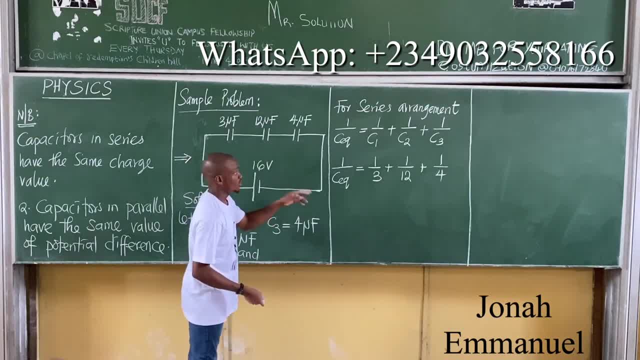 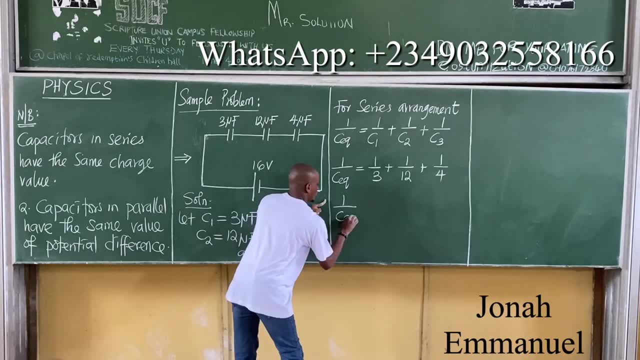 is because the units are the same. If your units are not the same, please convert first. So I'm having one over CEQ, This one here, three, twelve, four. My LCM is twelve Twelve over three, four times one, four plus. 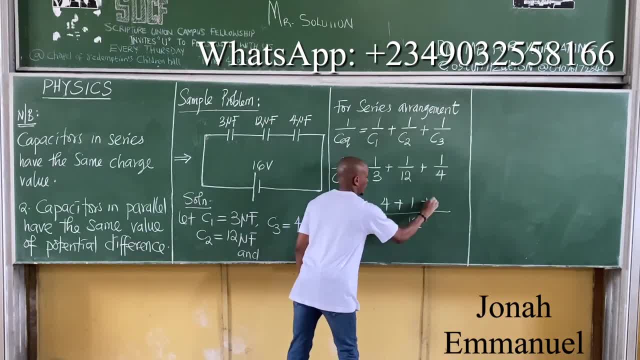 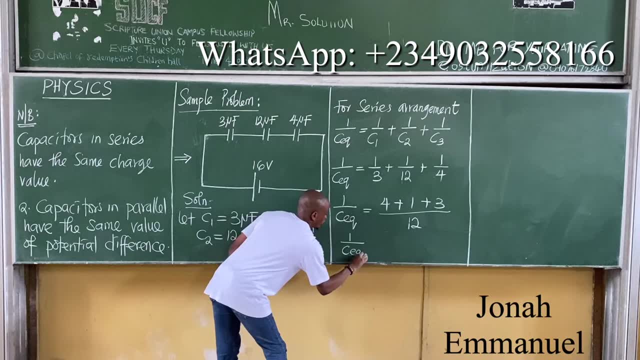 Twelve over twelve, one times one, one plus Twelve over four, three times one, three. So I have one over CEQ equal to this, this, this Eight One over twelve. Reduce the lower stand, Two here four. 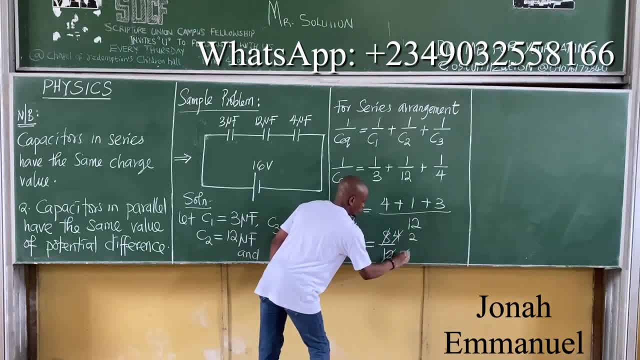 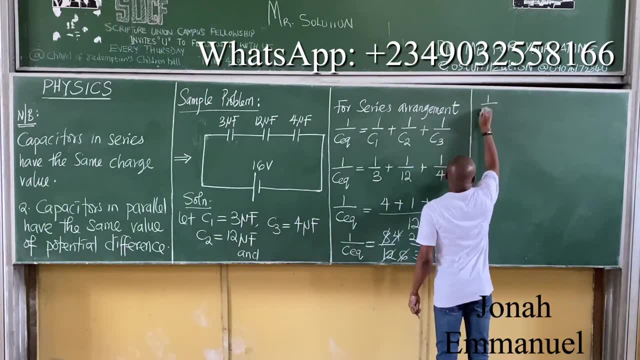 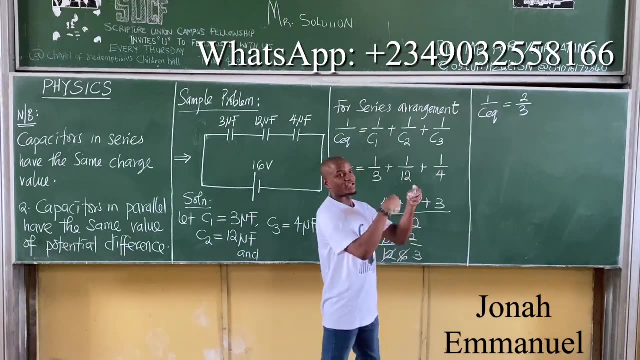 Two here six, Two here two, Two here three. So I have two over three as this. So it means that one over CEQ is equal to two over three. To get your equivalent we say INVAT. So INVAT is I have that CEQ all over one. 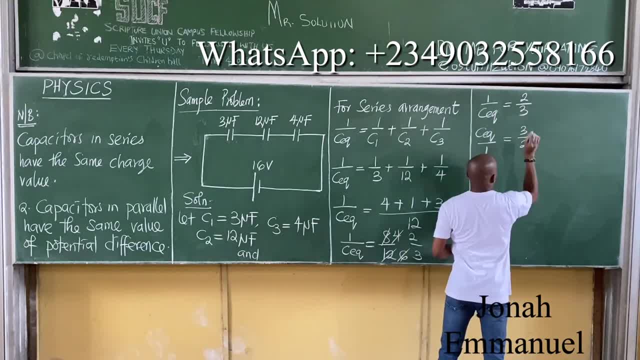 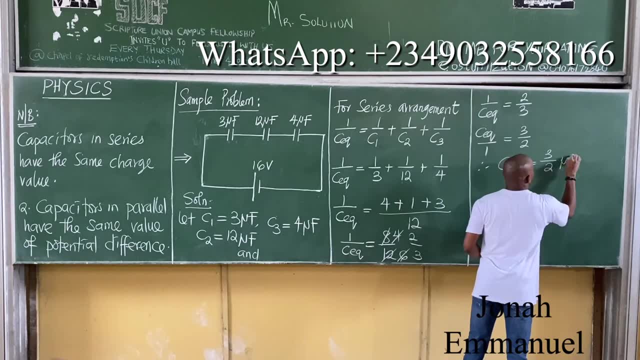 is equal to INVAT is three over two. So therefore, my equivalent capacitance is equal to three over two microfarads. If you want to express it this way, I have that equivalent capacitance is equal to 1.5 microfarads. 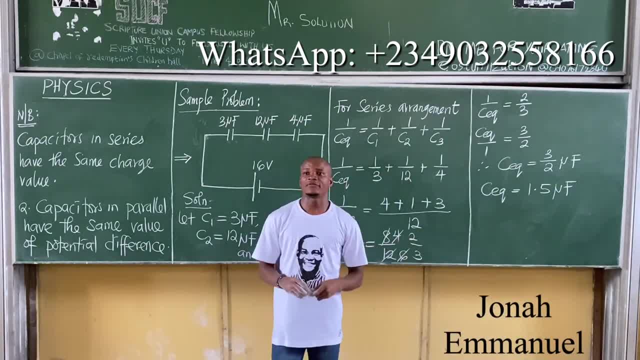 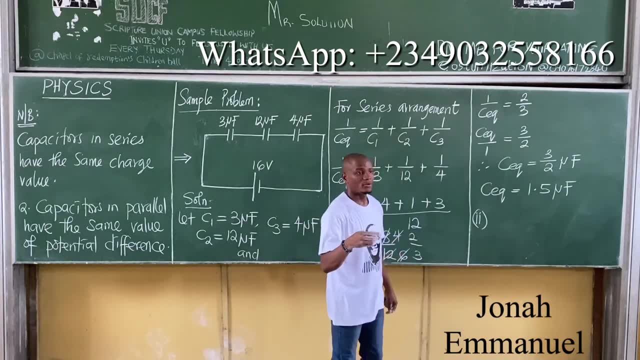 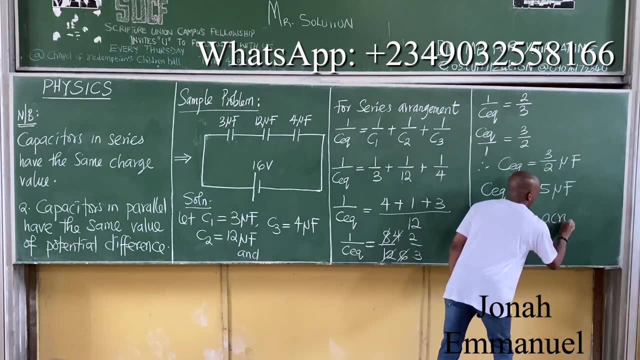 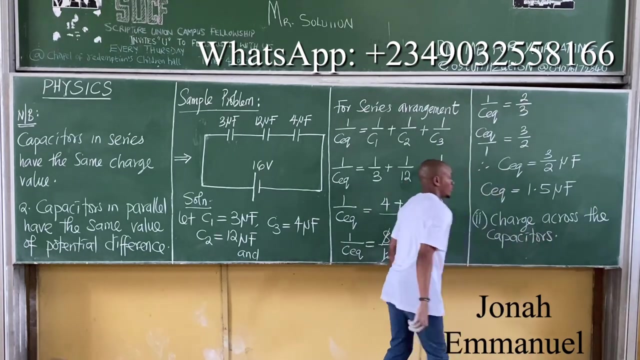 This is part one of the question. Part one says: find equivalent Equivalent capacitance. Part two says: find. what do you mean there? Charge, Let's get the charge, The charge across the capacitor. Now listen up. Listen up. How do you get charge? 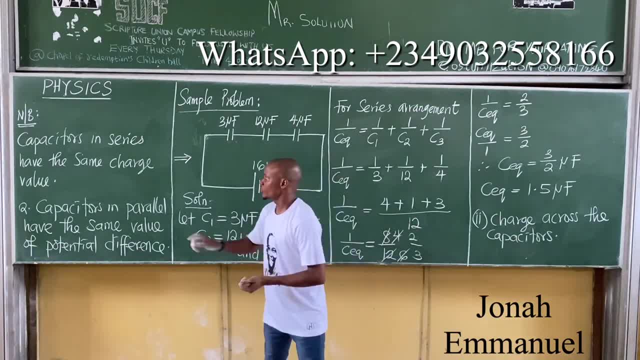 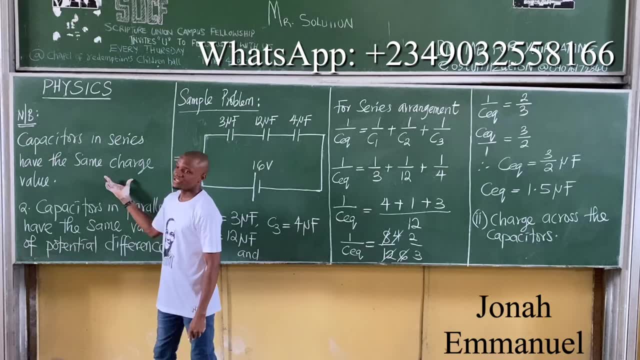 Listen, Listen, Before you get charge. fall back to this condition here, Please. Condition says that if they are in series, they have the same one there Charge value. if they are in series, If they are in parallel, they have the same potential difference. 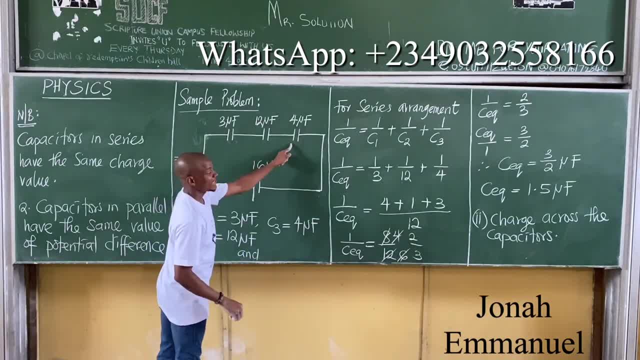 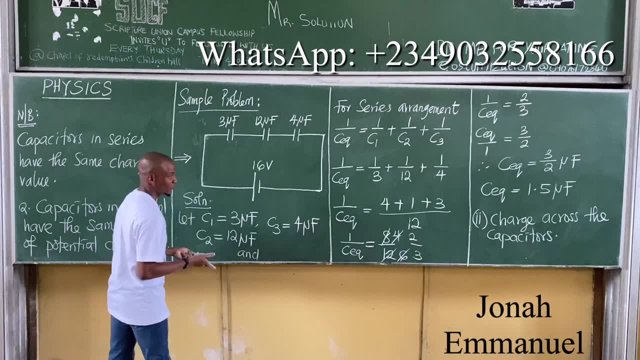 Obviously from my arrangement. here my capacitors are in series, So what does it mean? here They have the same charge value. So question: what's the charge value? I will go back to my initial equation. Recall something. Recall this. 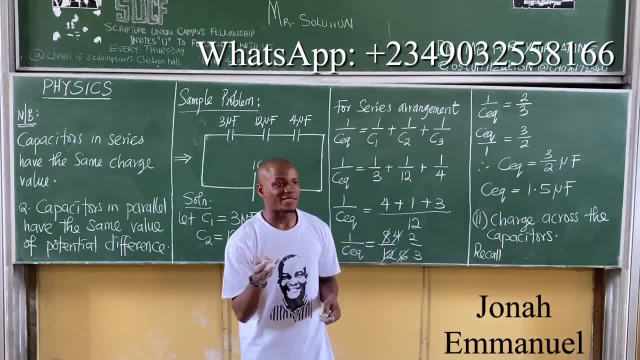 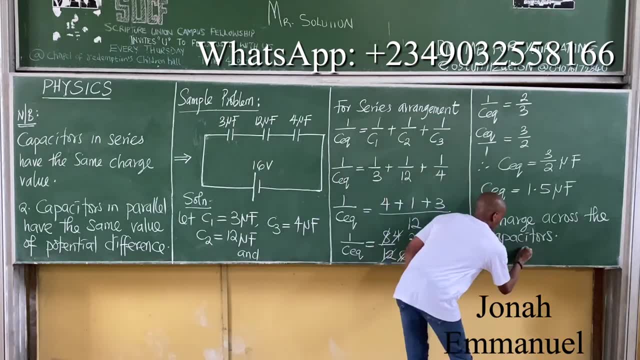 If I have charge Q, I have capacitance, C, I have potential difference V, What equation will it give them? Q is equal to what? there? CV, CV, All right, So U is to get the value of charge. 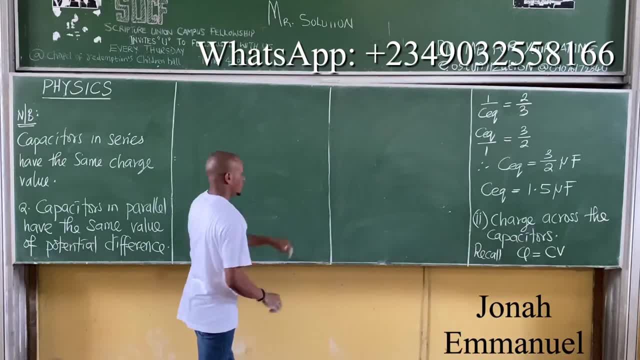 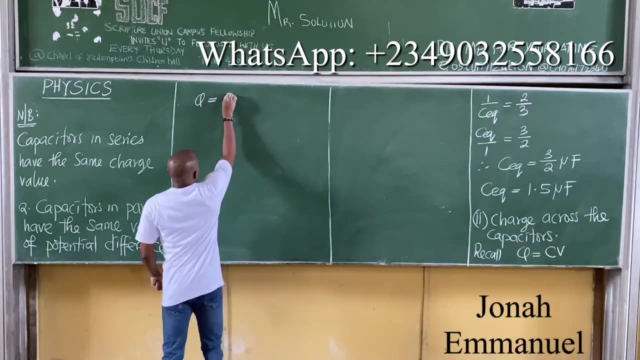 Now listen For this case, if you have that, C is equal to. now listen, Since I have multiple capacitors, since I have multiple Q, is equal to what there C equivalent times V. So you have V, All right. 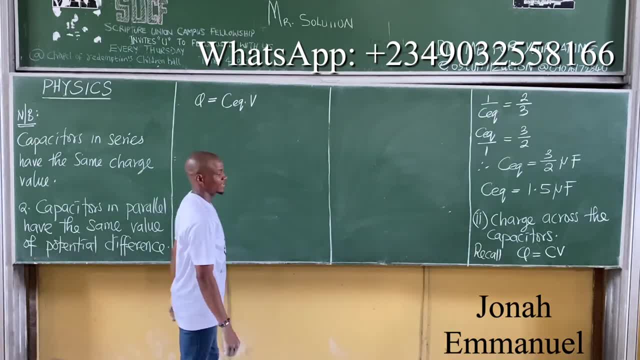 U is equivalent to V, Since you have multiple capacitors. So for this I have that Q is equal to. this is 1.5.. 1.5 of Z is micro, So it becomes 1.5.. 1.5 times 10 to the power minus 6.. 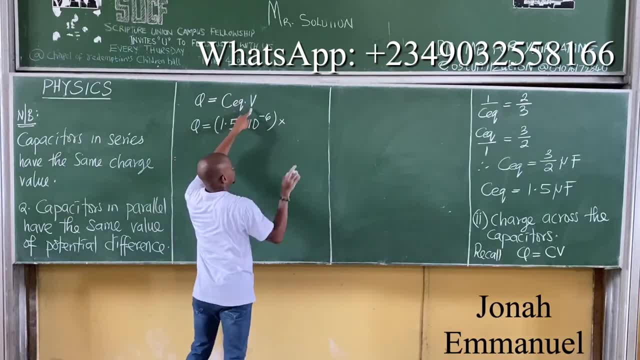 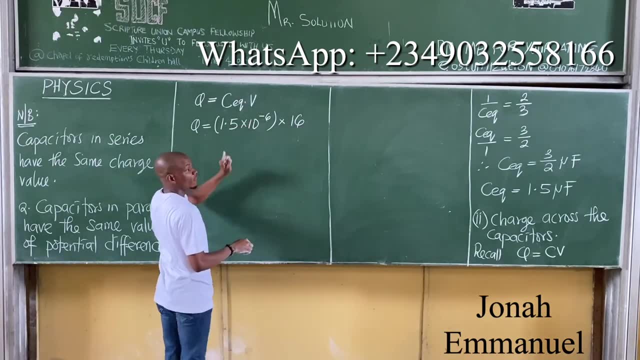 That's this equivalent times. please check Your voltage. was what there? 16. How many, 16. 16. 16, how many Volt? So volt means I'm not converting If it was 16 millivolts. 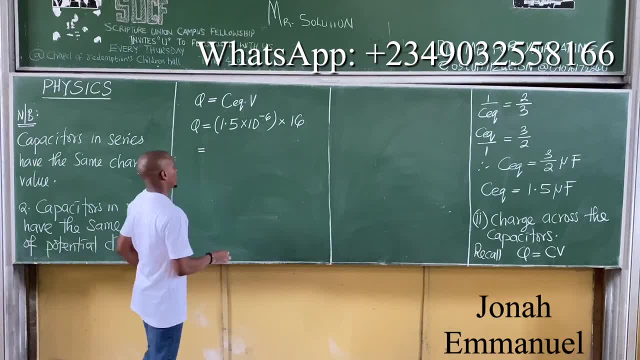 you know what to do. All right, Please, you've got to tie this where you are. Please. what? What do we have? 2.4 times 10 to the power minus 6.. 2.4 times 10 to the power minus 5 units. 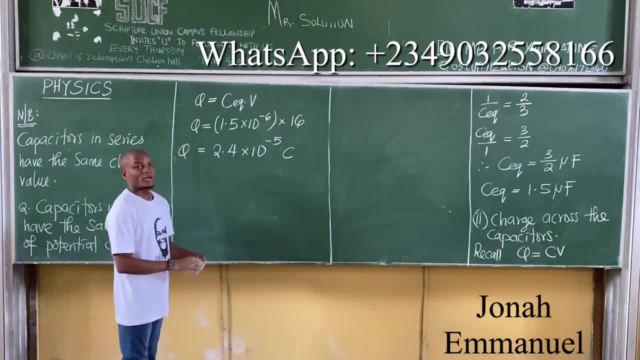 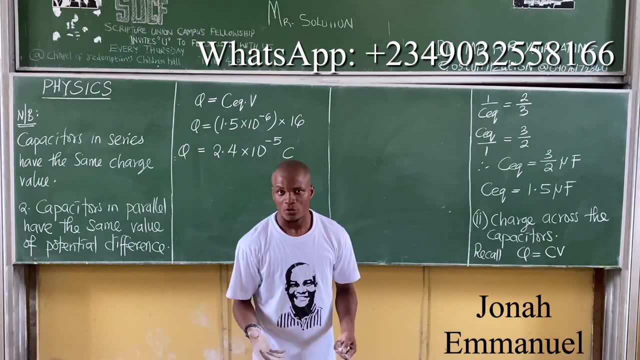 Units: Collie, Collie. All right, Listen, I wasn't asked to find the charge. I was asked to find out there the charge for each capacitor. That means from here. I was asked to find the value of Q1,. 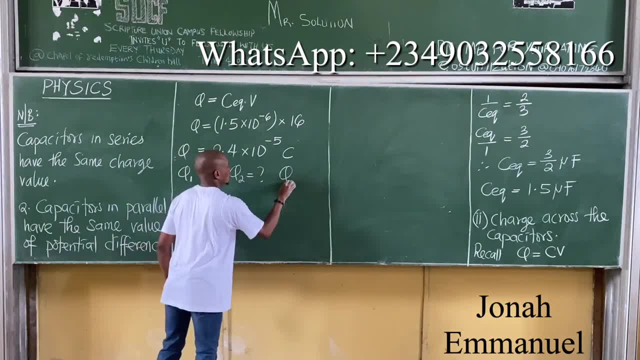 Q2, and Q3.. Find the charge for each of them. Now here's my condition. We said, since they are rated 6,, what would they allow? They have the same charge value. So therefore it means that Q is equal to Q1. 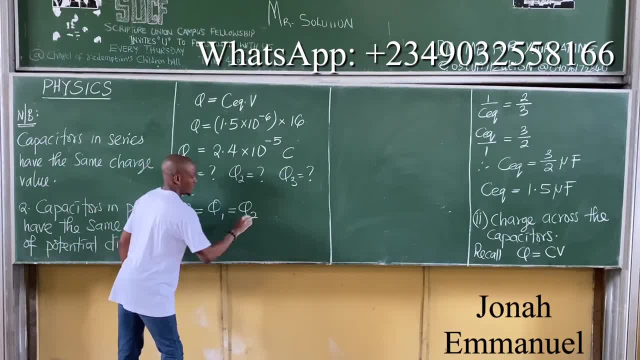 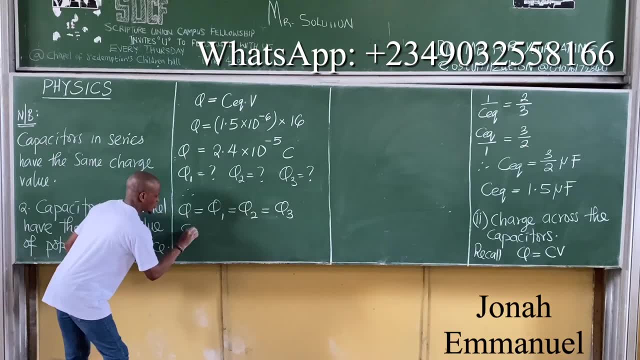 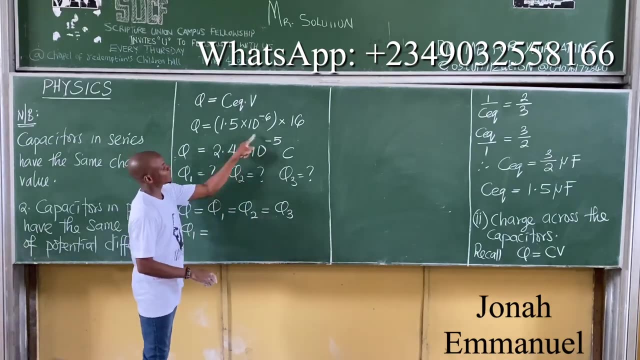 is still equal to Q2, is still equal to Q3.. The same charge value. Why See this arrangement? So, therefore, it means that Q1 is equal to this value. For physics sake, can we express this in terms of a prefix? 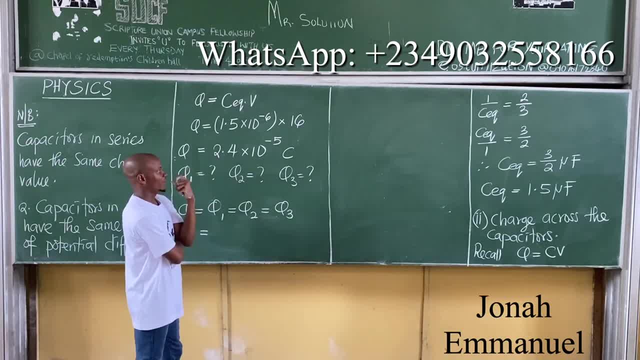 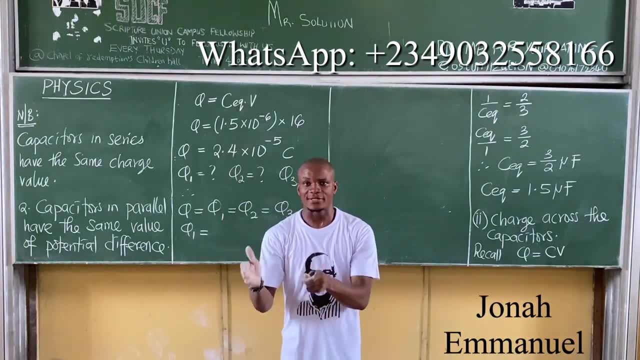 What would it be? Can we express this in terms of a prefix? What would it be? Note that your prefixes are in threes Milli mega. whatever They are in threes, That's 369 minus 3 minus 6 minus 9.. 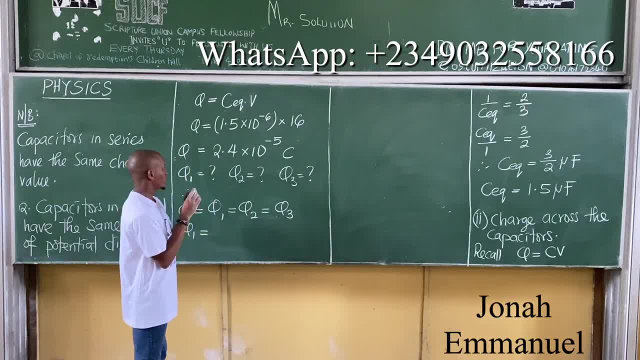 So express this as a prefix. What would it be? No, No, To make this my micro. I might multiply by 10 or divide it by 10.. Huh, This is minus 5.. Let's say I want to make it minus 6.. 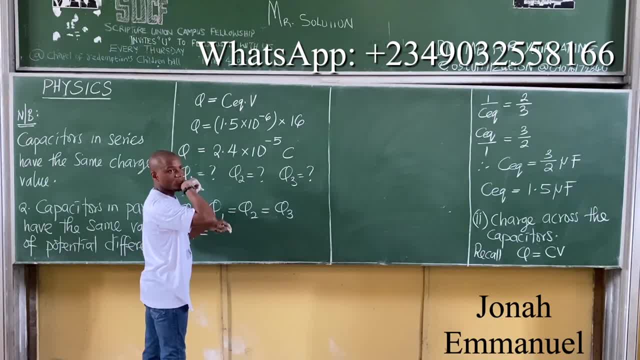 Would I get to leave it 0.24 or 34?? Obviously, If I want to make this minus 6, I have to move it this way, So it becomes 0.24 times the power there minus 6. So it becomes. 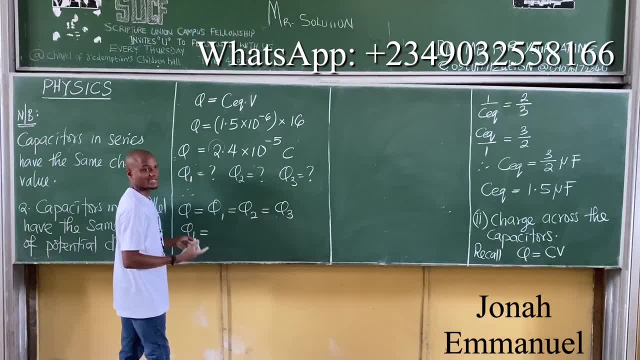 0.24 micro-poly. That's it In the term. you're dividing by 10, not multiplying Alright, But that's by the way. So we can say this is 2.4 times 10 to the power, minus 5 poly. 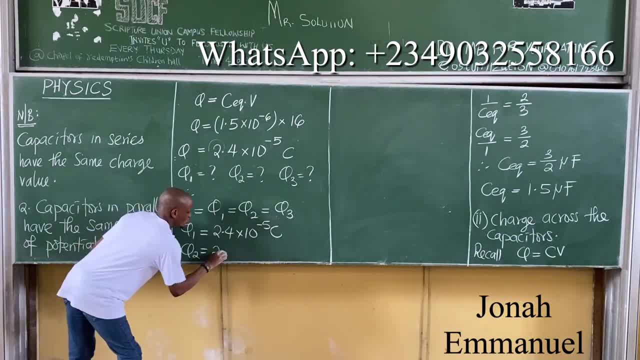 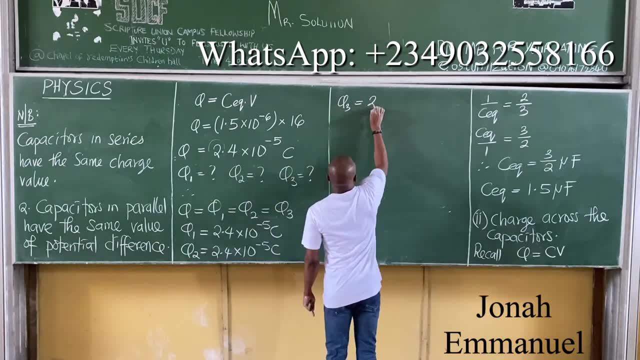 It's still okay. Q2 equal to 2.4 times 10 to the power minus 5 poly, And then Q3 equal to 2.4 times 10 to the power minus 5 poly. So I have this: 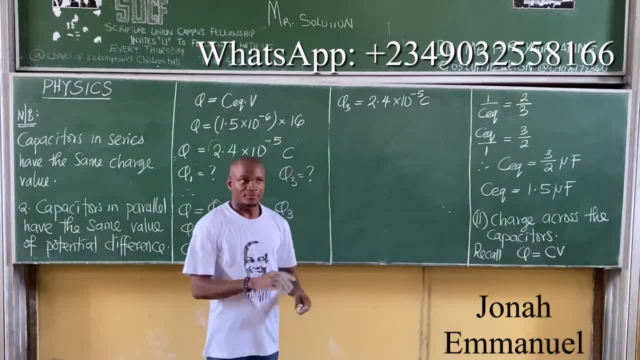 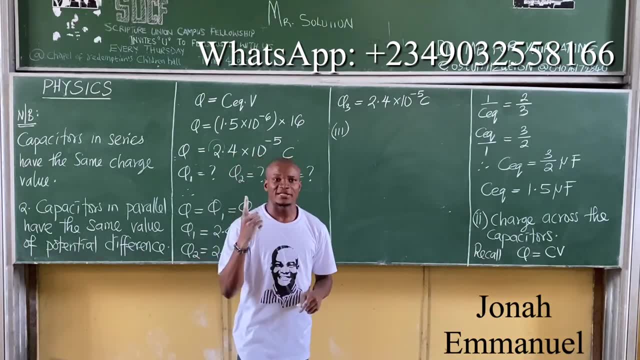 Alright, This is this The third part of the question. Now Q65,. number one: equivalent capacitance. Number two: the charge across the network. Number three: the potential difference across the network. Now, listen, Listen, It was a series arrangement question. 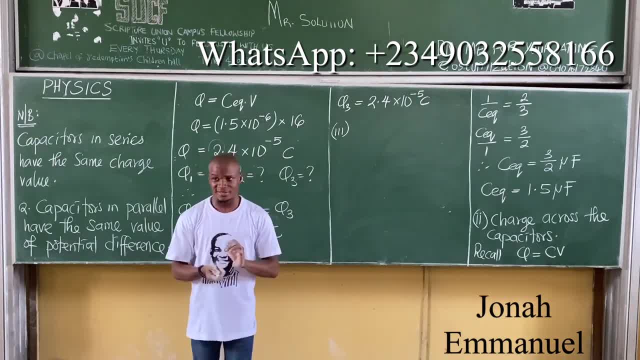 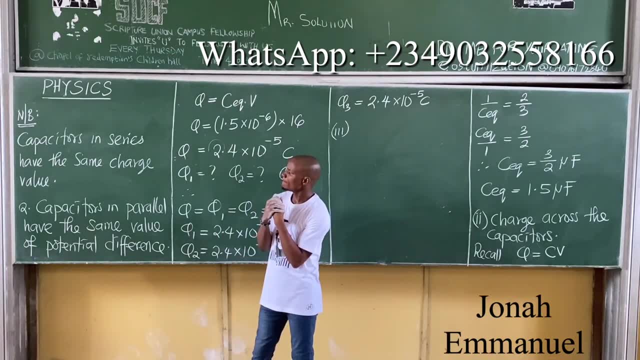 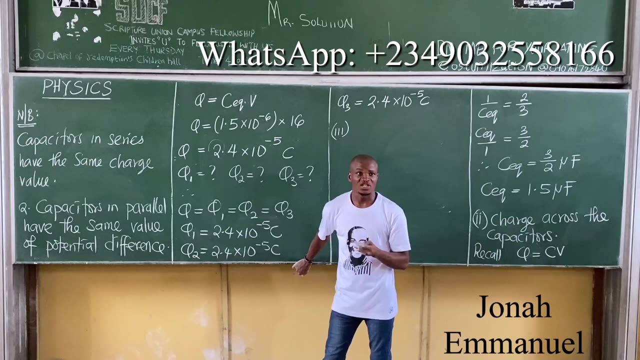 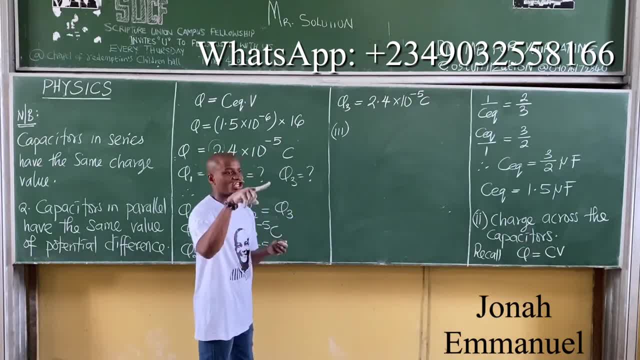 is Well. the charges were the same For series arrangements. the potential difference is not the same. They differ, Please My. my tip is now to get potential difference. please check your formula. We said V is equal to what there. 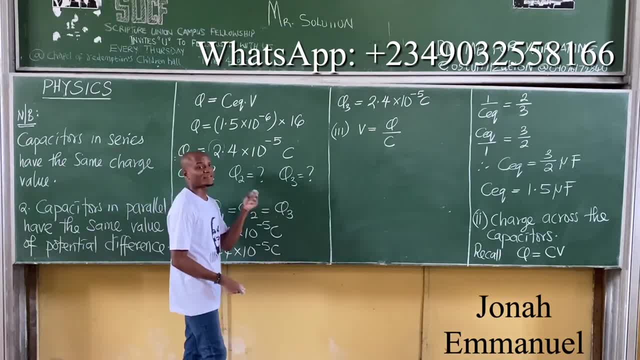 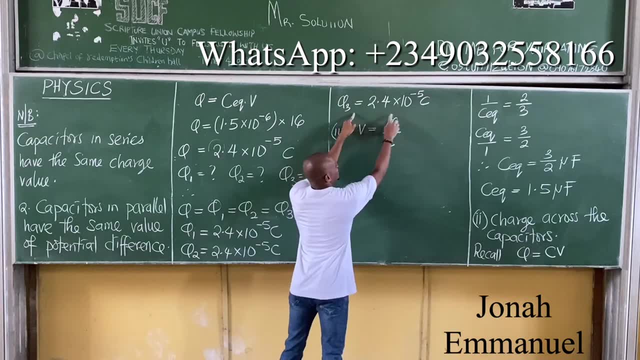 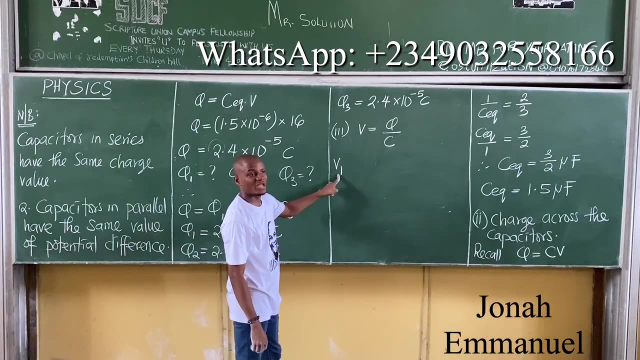 Q, our words Z. So if you've gotten the charge for each of them- Q1,, Q2, Q3.. My tip now: So for this one here- now, here's my home black holes- let's get B1.. So the potential difference on your C1 capacitor is equal to Q1 on the water C1.. 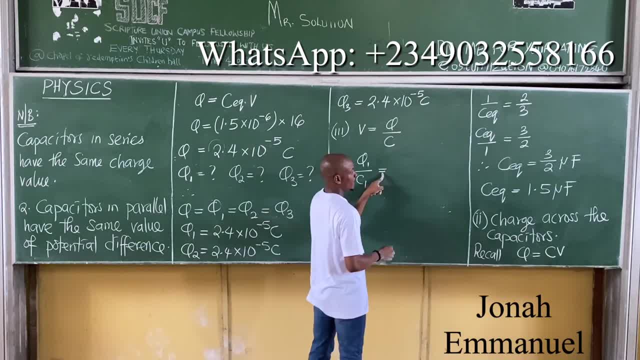 Now that's equal to: please give me Q1 again there. what do you have? Q1, sorry, 2.4 in micro micro. sorry, this one again, 2.4 times 10 to the power minus 5, all over. give me C1, please. 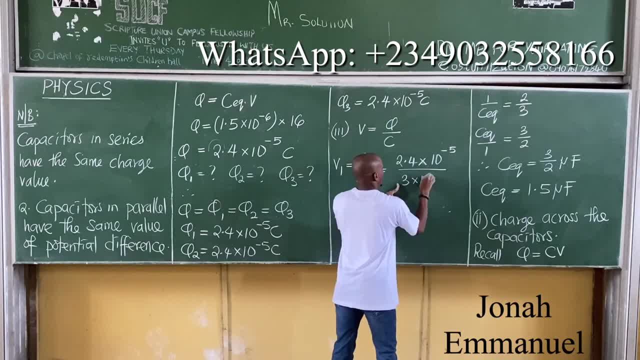 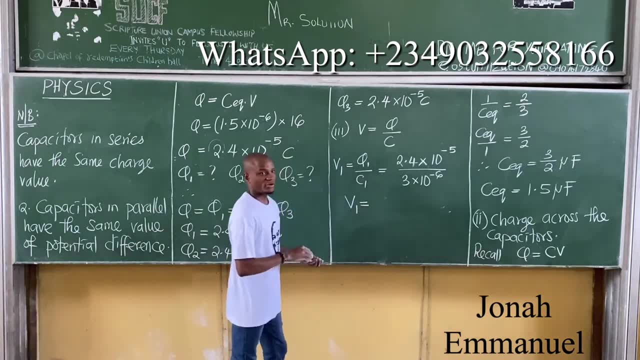 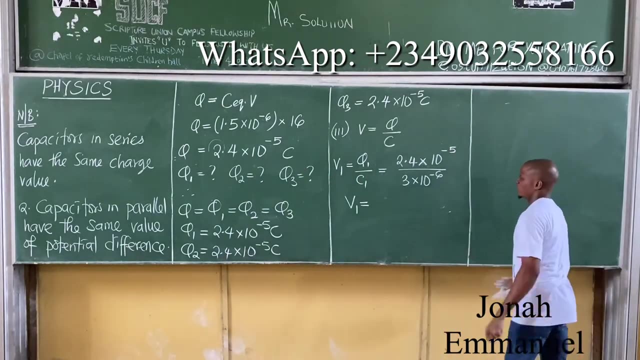 3 minus 5, 3 times 10 to the power Minus 6,. please point this correctly. what's your value? Point this correctly, please. what's your value? Please point this correctly. what's your value? 8 volts. 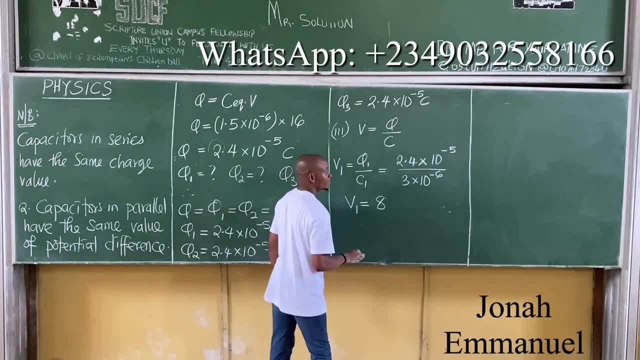 Huh, 8 volts, 8, 8. what 8 volts? Right, Let's get V2.. V2 will be equal to, from the same concept, Q2 over C2.. That's equal to Q2 is a constant same thing here. so 2.4 times 10 to the power minus 5,, all over C2, please recall C2. for me, 12, right. 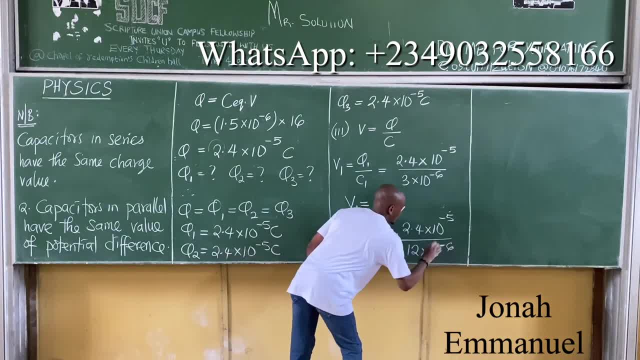 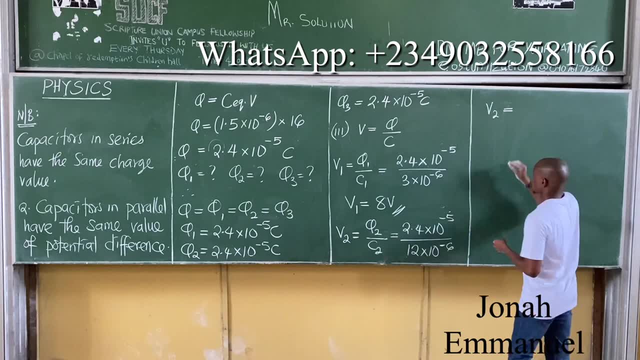 12.. So 12 times 10 to the power minus 6, 12 micro. So I have that V2 is equal to how many 2. 2. 2 volts, 2 volts, Finally, V3.. 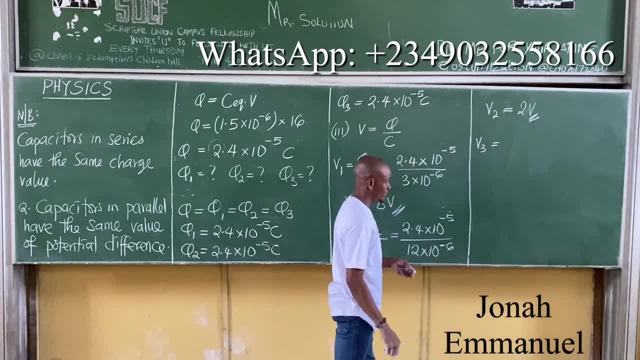 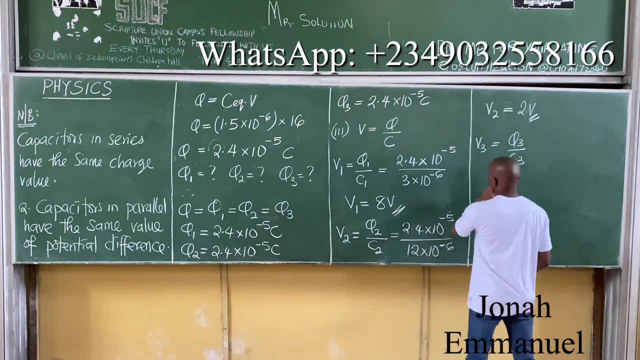 So the potential difference on the third capacitor, V3, is equal to Q3 over C3, and that's equal to Q3. is how many there? Same thing here: 2.4 times 10 to the power minus 5, all over C3 was what. 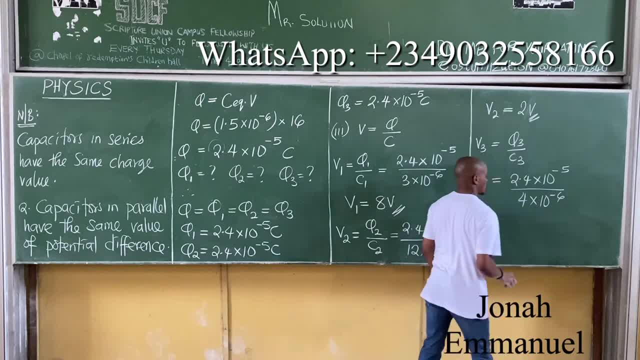 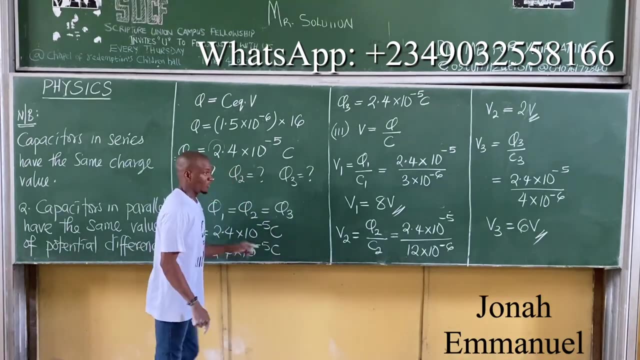 4. 4 times 10 to the power minus 6, 4 micro. That means V3 is equal to how many 6. 6 volts. So here's your thing. For series arrangement of capacitors: they have the same value for charges but different value for what. they have potential difference. 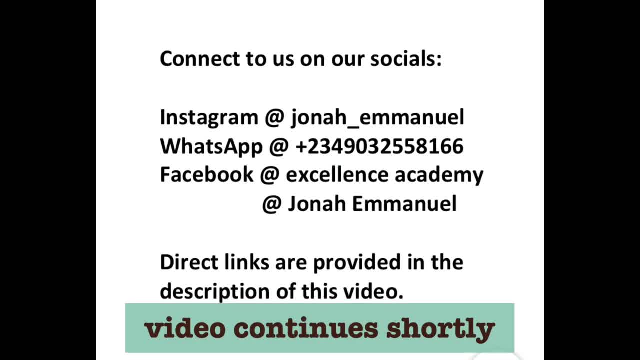 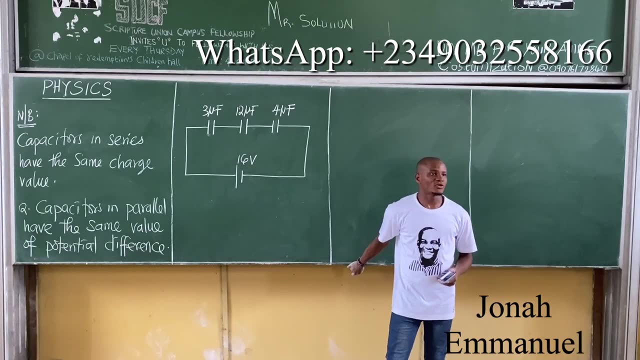 That's it, guys. Look at this. One last thing on this. One last thing. Okay, wait. One last thing on this, please My Listen, Listen. If I look at the concept of capacitors, I have only three parameters. I place majorly. 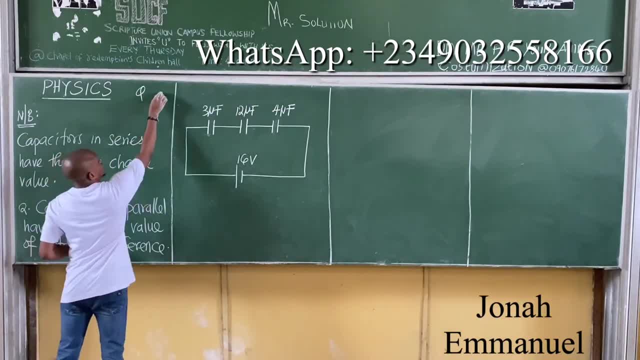 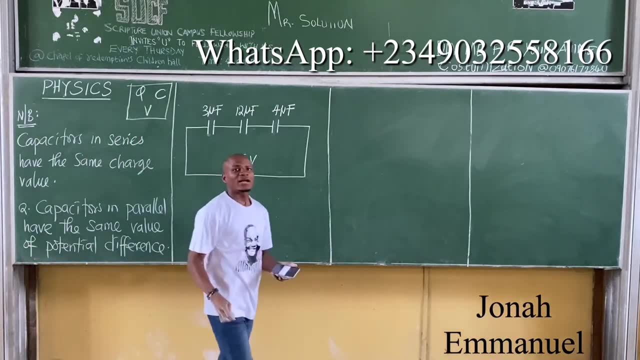 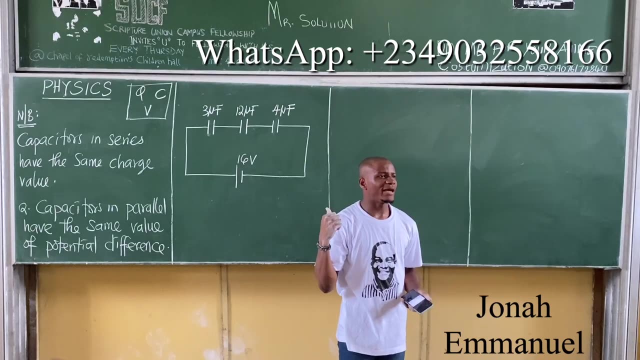 That's your charge Q, Your capacitance C And your potential difference V. These are like the three things I do, Of course here. can I introduce current to this: How? What's the formula V1 to IR? 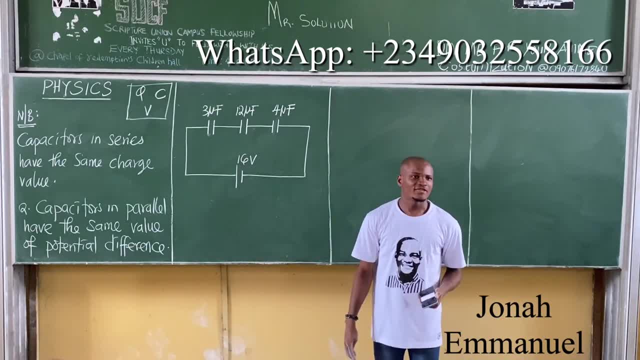 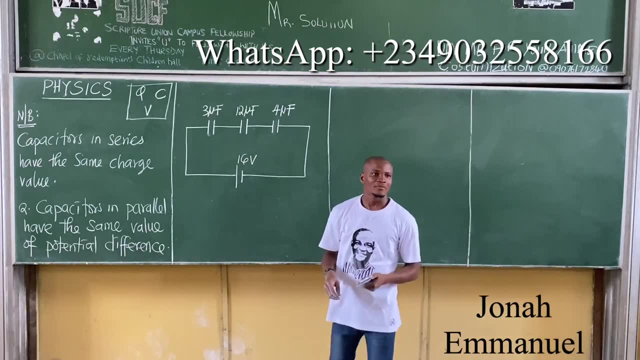 where's the R from here? if you say I R, where's R here? where's resistance here? V equal to I R, that's Ohm's law, no problem. but where's the R? there's no resistance here. so if you say V, 16 equal to I. 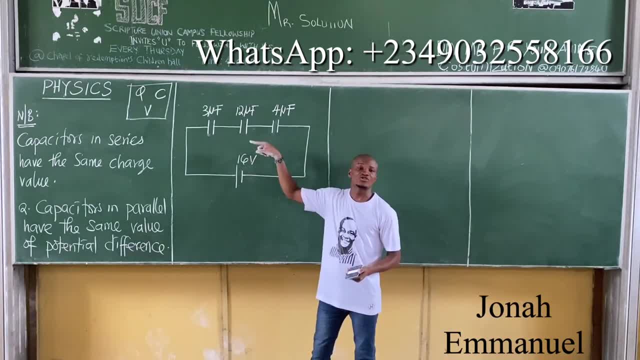 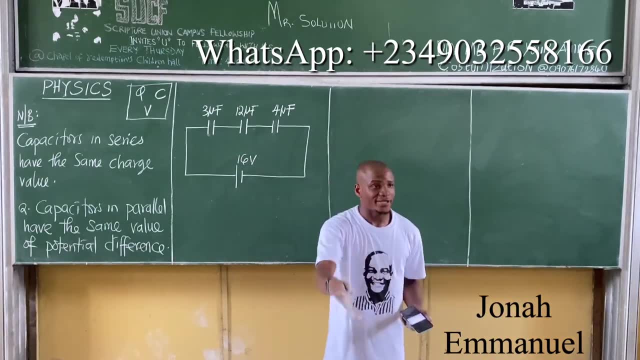 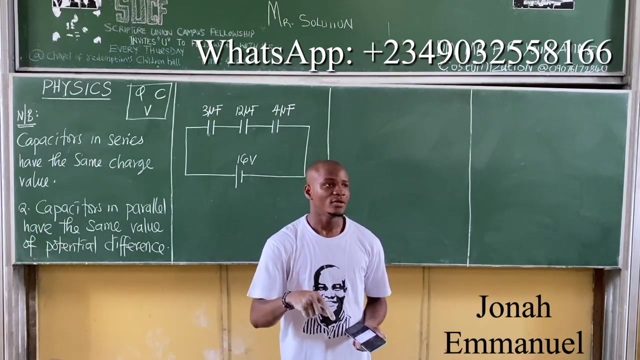 there's no I here R resistance. you're only with two unknowns, which is not possible. so how do I introduce correct to this? because in the exam they ask to find correct? how do you find correct? take down this. take down now. listen. listen. V equal to I? R is Ohm's law. 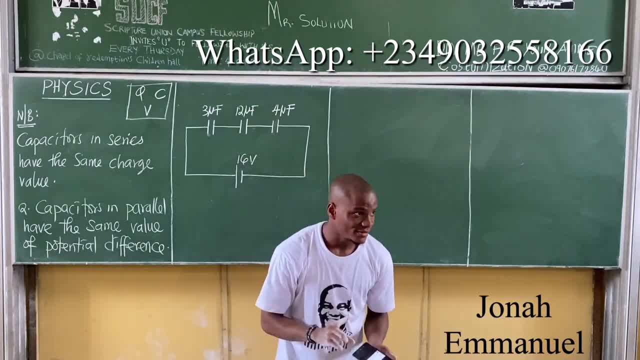 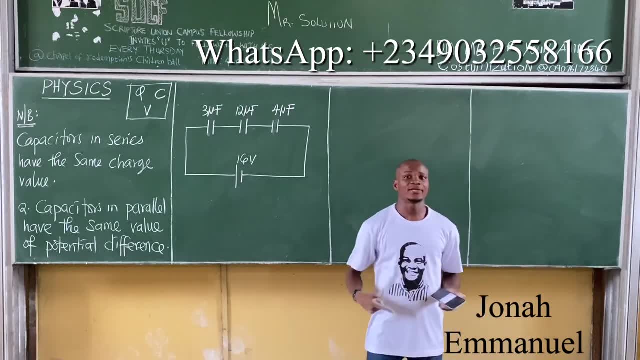 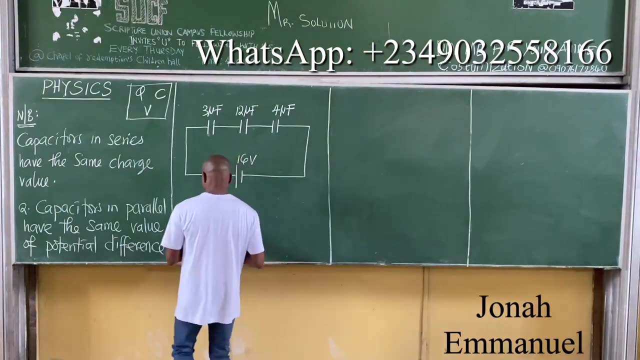 under the resistor arrangement. for capacitor arrangement like this, there is also another form of Ohm's law for this. take down this Ohm's law: input for a capacitor is given by Ohm's law for a capacitor is given by I equal to C divided by T. 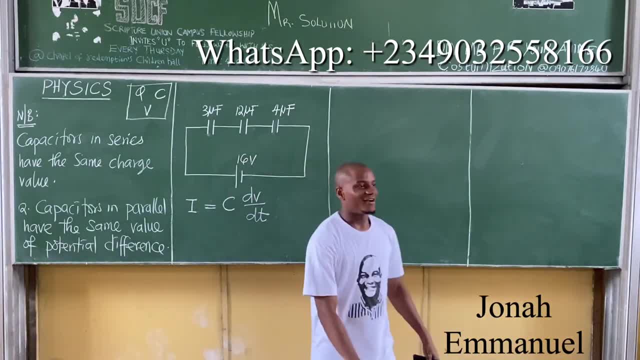 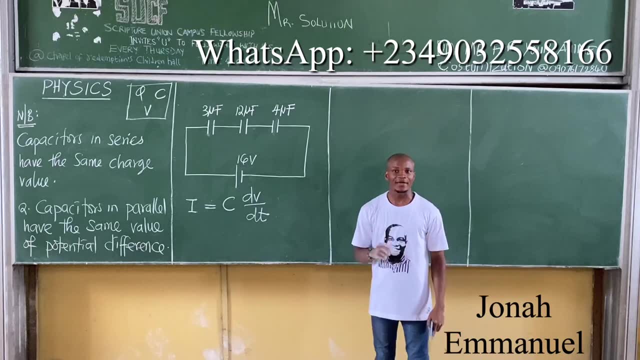 I'll come back to calculus. Ohm's law for a capacitor circuit is given by I equal to C divided by C over T. so you know what that means. is that right? if they give you the potential difference in terms of time, you differentiate. but don't worry. 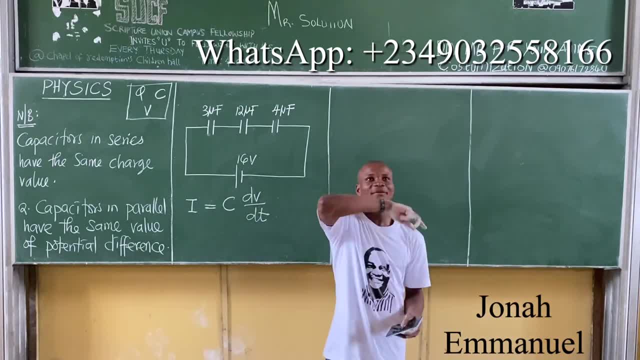 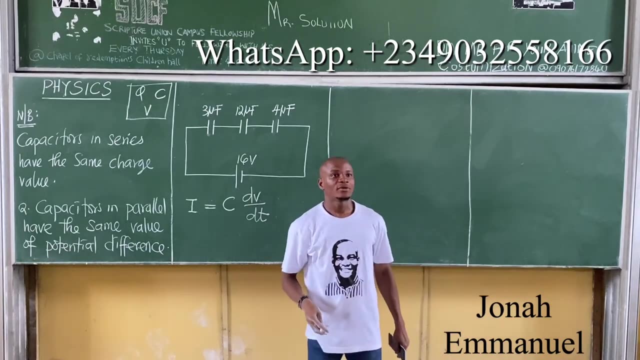 this one is not maths. they won't give you the equation, they'll just say: find the correct at so so. so, second: ok from your question. take down we've done. I, I, I, I, I take down this. I V, I V find the current in the circuit. 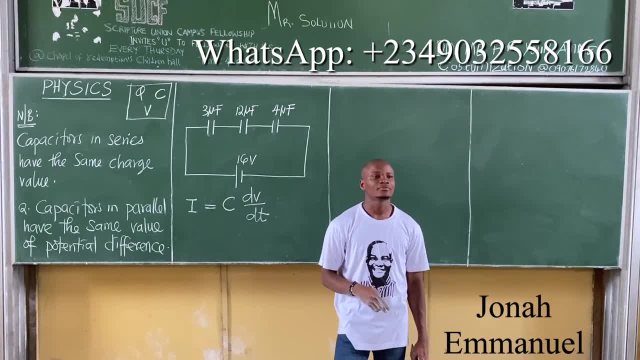 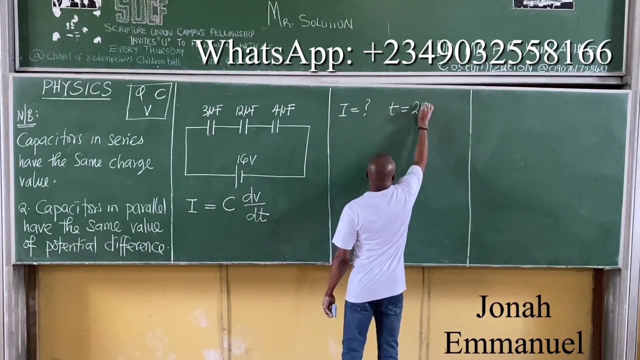 find the current in the circuit after finding. find the current in the circuit after twenty seconds. find the current in the circuit after 20 seconds. we have to find I after T, equal to 20 seconds. For this case. look up For this case. it's as easy as this. For this case. now, please check. We have equivalent capacitance to be how many 1.5 microfarads, So we have to find correct. 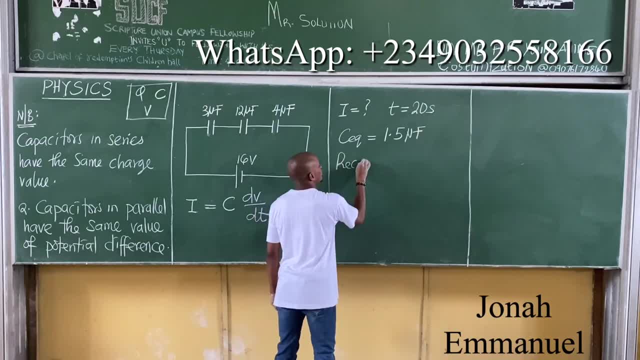 So for this one I'm now saying: recall, Recall that Ohm's law for a capacitor setting is: I is equal to C, the V over the T In this case, what we do is simple: It's now equal to. this becomes not just similar, but equivalent. 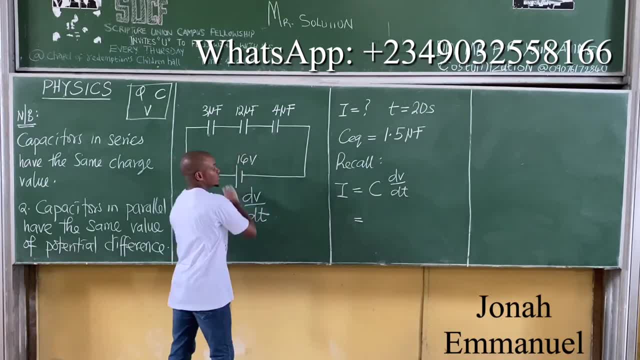 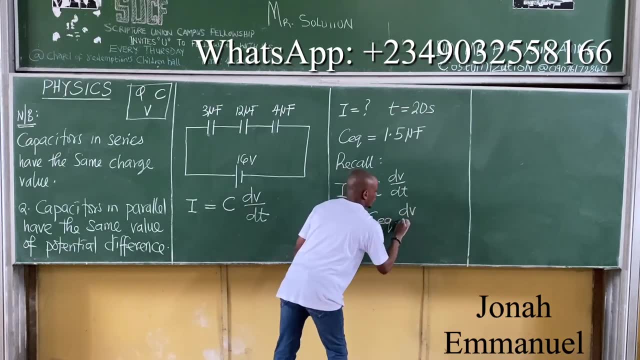 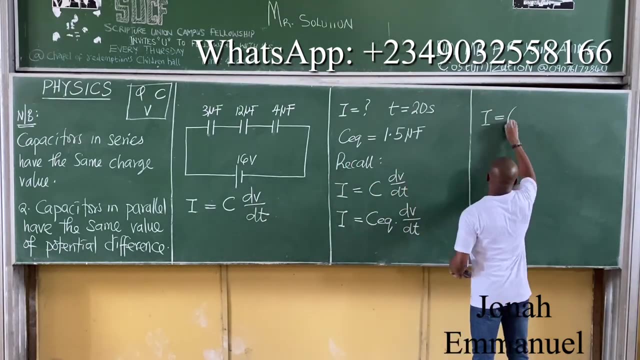 Since I have several capacitors: 1,, 2,, 3.. So I will be equal to the equivalent capacitor. Then the V all over the T, Hence I will be equal to. equivalent- is 1.5 times 10 to the power minus 6.. That's micro multiplying the V over the T. 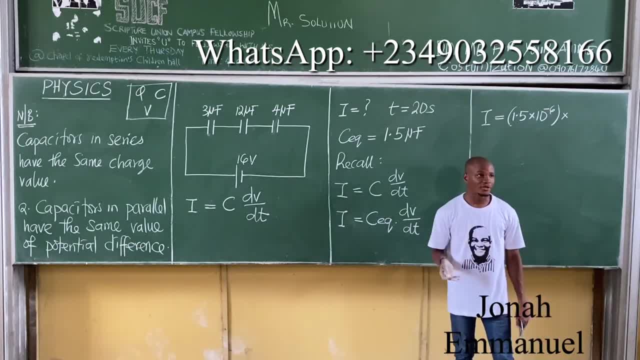 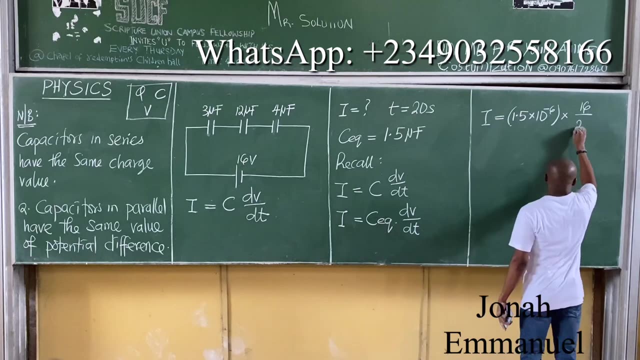 Now for this one here. don't really bother about differentiation because you're not given an equation. Just put one there: V over T. What's V there? 16 volts, It becomes times 16 all over T. See the time That's 25 volts, It becomes 20.. 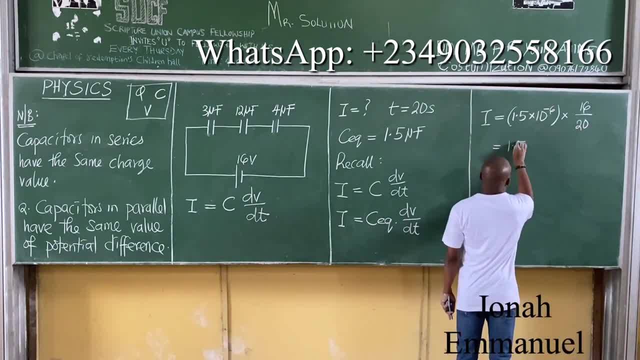 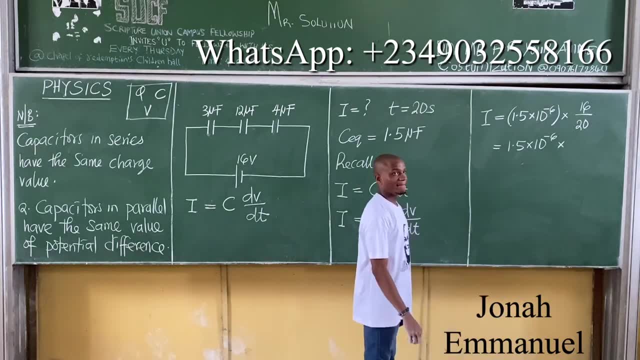 So that's equal to 1.5 times 10 to the power minus 6 multiplied. Please, what do you have here? 6 over 20.. What do you have? 0.8. 0.8. 0.8.. Please, multiply. for me, I is equal to what do I get?